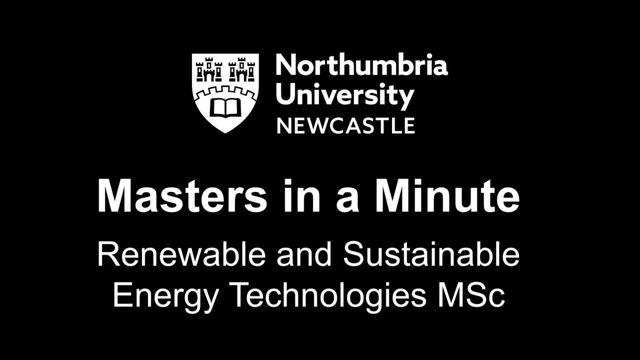 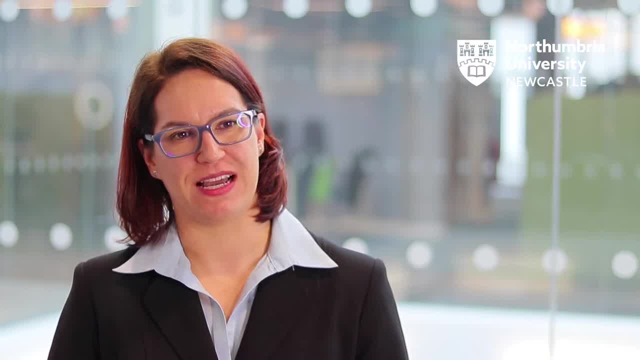 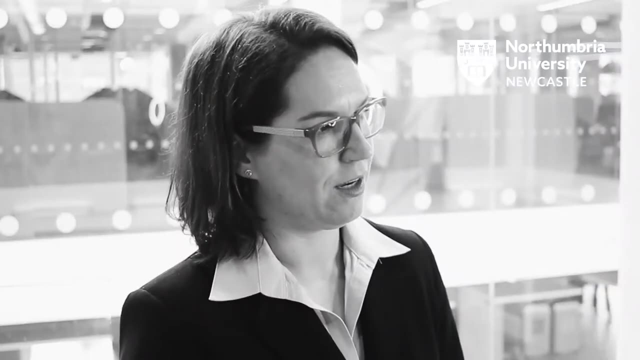 Hello, my name is Madeleine Kombrink. I'm a Senior Lecturer in the Department of Mechanical and Construction Engineering at Northumbria University. I'm here to talk about our MSc in Renewable and Sustainable Energy Technologies. Our course in Renewable and Sustainable Energy Technologies is fully accredited by the Institution for Mechanical Engineers. 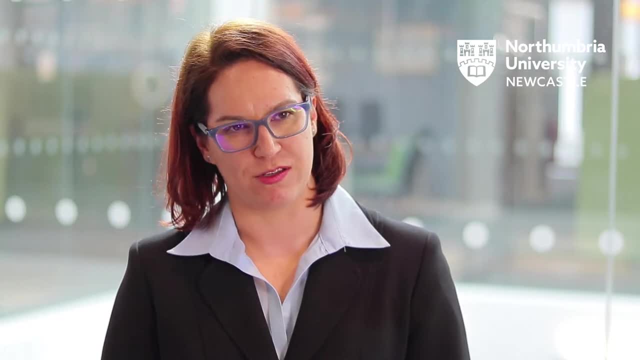 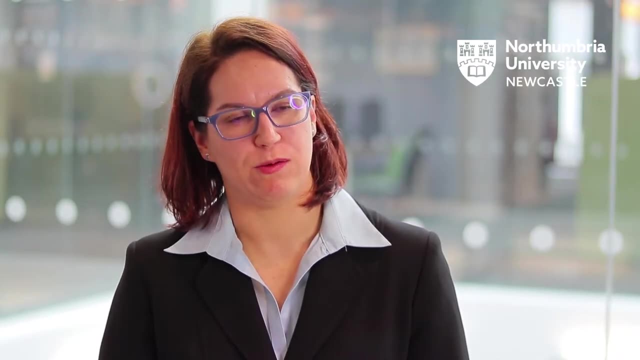 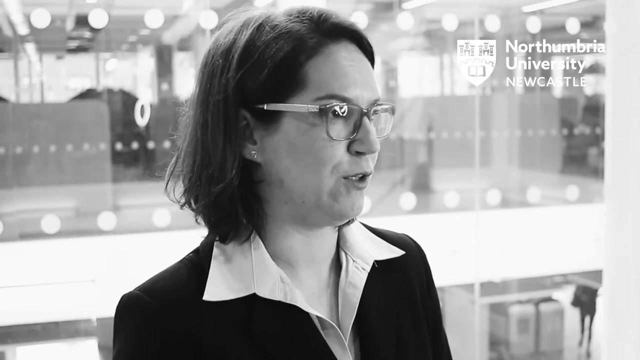 Our programme is structured into two parts. The first component consists of coursework and the second of a research project. During the coursework, you will become skilled in the subjects related to energy management, such as energy conversion systems in photovoltaic cells, wind generation and ocean energy generation. 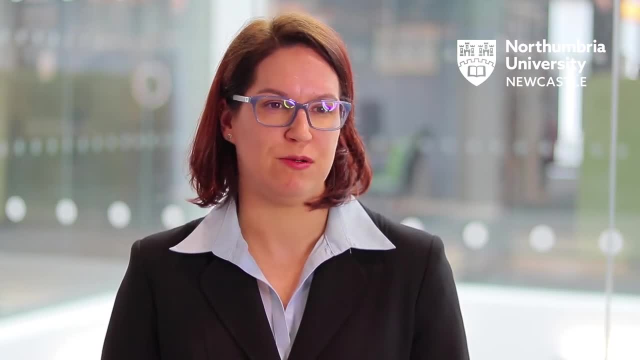 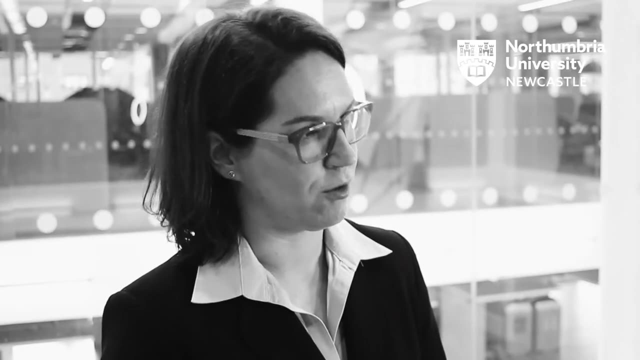 Furthermore, there are subjects related to building modelling and design optimisation. After completion of the coursework, you will engage with a research project. There will be a member of staff who is an expert in the field of renewable and sustainable energy that will guide you through this process. 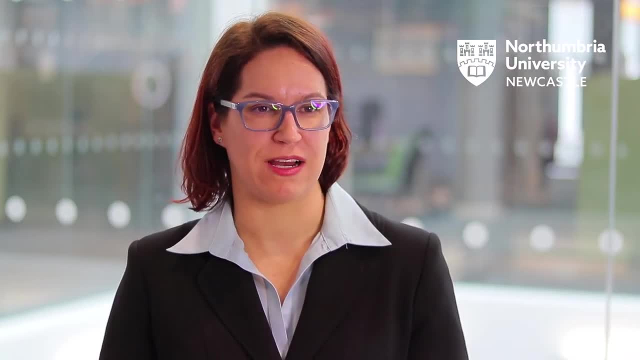 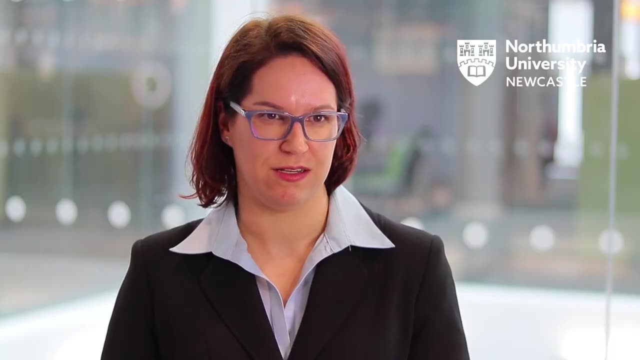 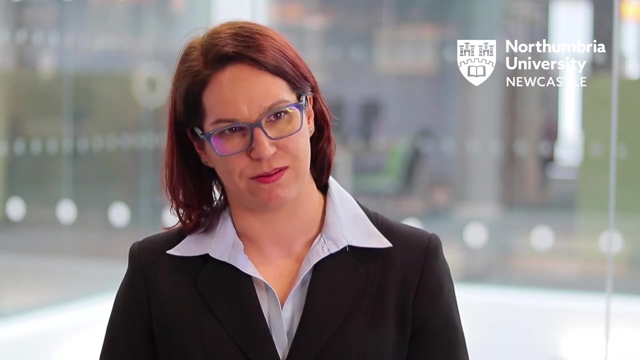 The university has a well-established track record in the field of renewable and sustainable energy research. We have strong links with industry and this is to the benefit of our students, as they get to engage with the latest technologies and methods in this area. Thank you. 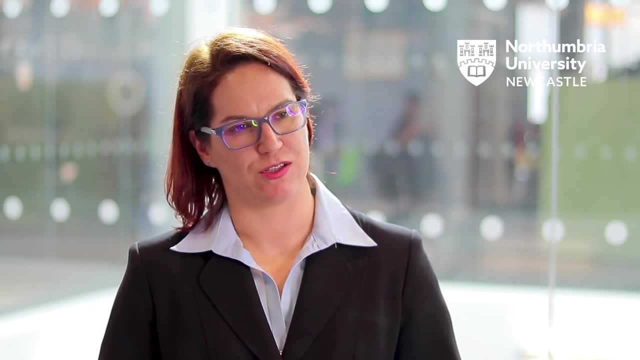 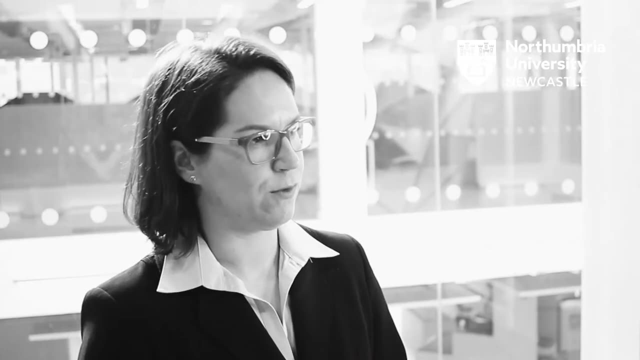 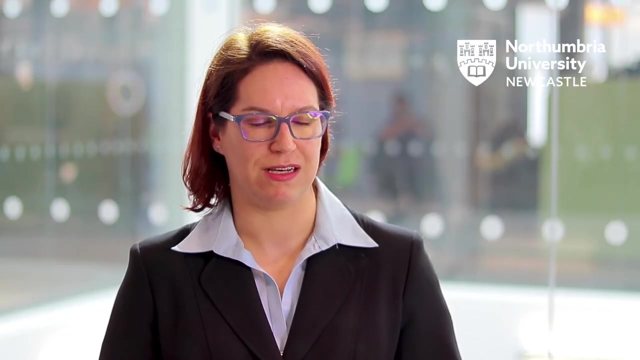 At Northumbria University. you will have access to software laboratories hosting the latest version of software used in industry today. We have the full versions of MATLAB, ANSYS, CATIA and other software. You will become skilled and highly proficient in the software, which will greatly enhance your employability. 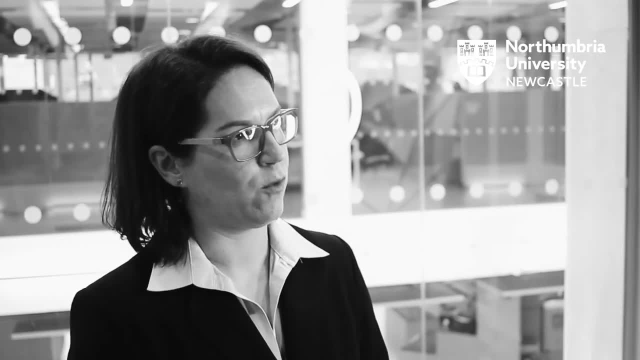 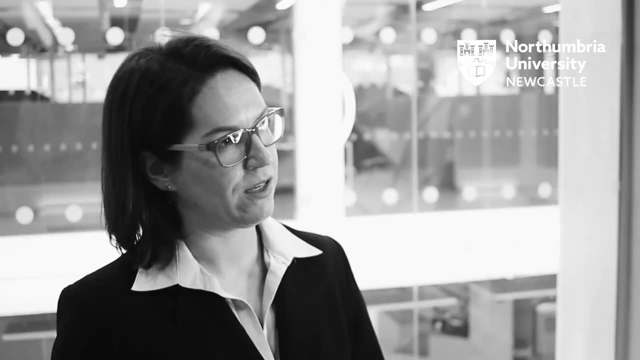 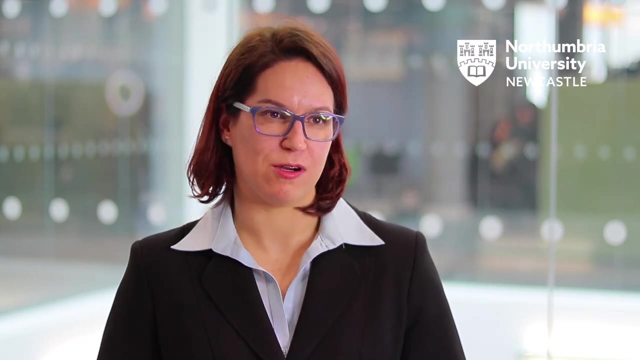 We have laboratories that specifically caters for wind energy testing, photovoltaic cells and battery testing for electric vehicles. You will become an advanced practitioner in the field of renewable and sustainable energy technologies. You can also have the option of remaining an academic and pursuing a PhD. 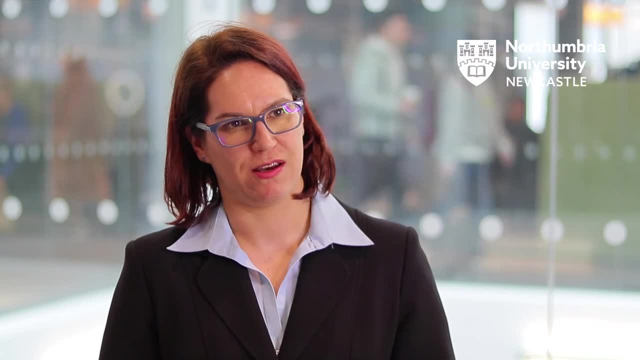 With the looming energy crisis at our doorstep, now is the best time to enter this dynamic field with our programme.